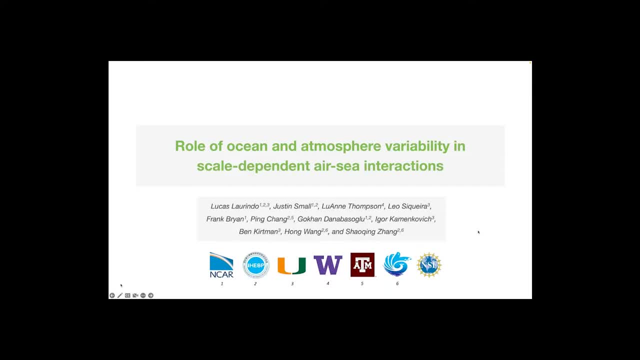 aerosol interaction. Today he will present to us one of his recent publications. That's my understanding, Lucas. Yeah, Lucas, welcome and take away, please. Thank you very much, Jimbo. Thank you very much for inviting me to be here. It's quite an honor. 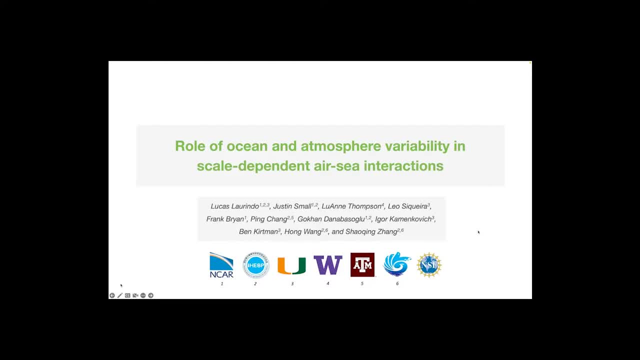 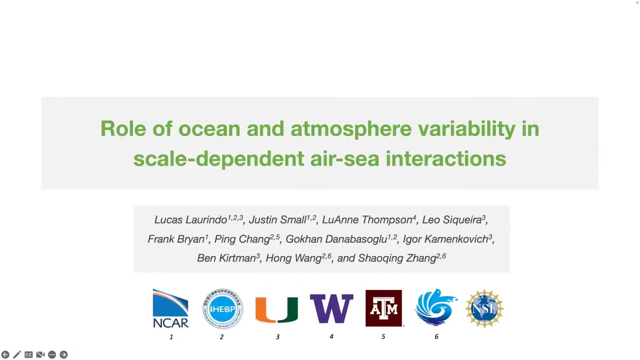 And the title of my talk is Role of Ocean and Observability Still depend on interactions. Let me share. Thank you very much, Thanks. Okay, is that the right screen? Yes, it looks good. Okay, thank you. Let's first acknowledge my co-authors, Justin Mouw and Louane Thomson, and sorry. 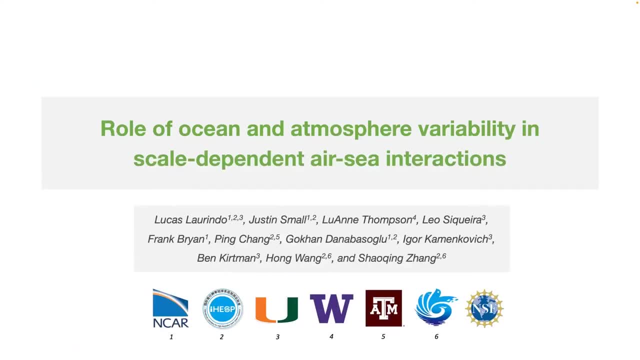 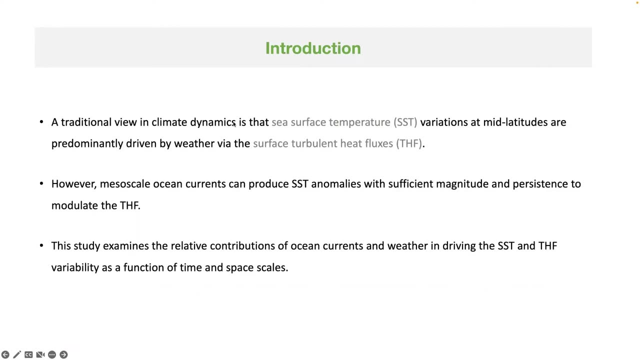 and others. I developed this work while I was a postdoc at NCAR And okay, uh, let's just start. uh, Um, I'm dynamics. Uh, we usually consider that the accessibility 3, the extra topic, is driven by whether the surface, uh, to make it plus, 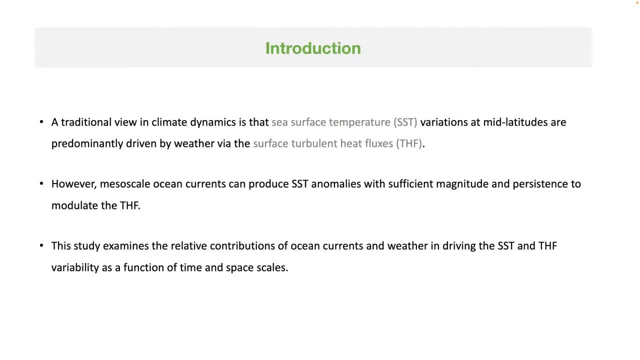 However, the best couple of decades. it has become clear that Metal scale ocean currents can also produce anomalies that are large and persistent enough To modulate the surface, and there's more and more evidence that this influence of uh the ocean 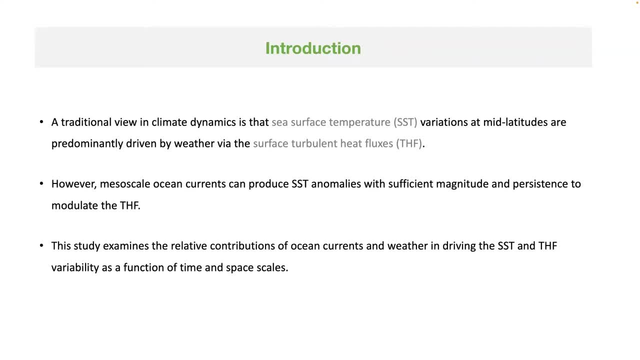 On the surface processes and play an active role in both weather and climate. So the main goal of this study was to determine the what are, Is the relative contributions of the ocean, and that was your dynamics for driving situations and situations in suffice. it looks as a facial time and facial skills. 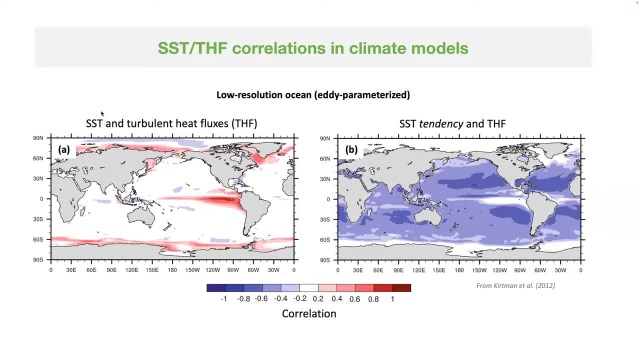 So I will start with maps- Uh, these are from Kirkman at all, 2012,- uh, showing correlations between: and the surface. Uh, and then obese. Uh, correlations between the rate of change. There's this tendency And the uh- these are from a low resolution is the model. 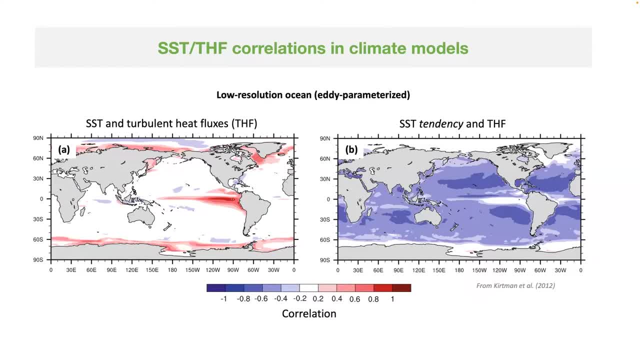 Uh, where the ocean that they will see are both configured to a 1 degree, For example, resolution, and these relationships can be used to infer the local of our abilities, driven mostly by oceanic dynamics. Named positive values- uh- indicate that the ocean cards generate the accessibility that, in turn, uh drives a response in the hip. 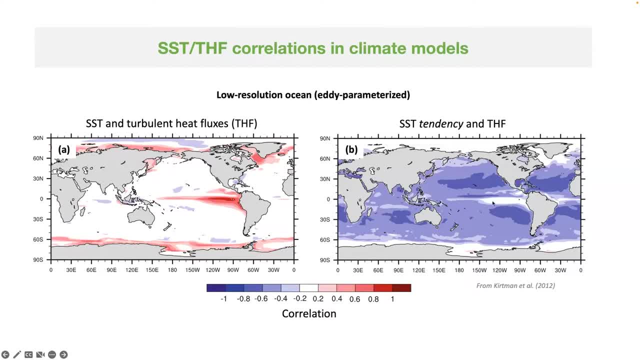 While in B Negative values, in the case that the atmosphere drive, there's just different situations, Eight to the heavier And in the case of the low res model, we can see the innovative correlations dominate almost everywhere except introduction. Sorry in the uh, sorry about these. uh, I think it's going to flip wholes for rapidly. The controls, your abilities sensitive. I apologize in advance. 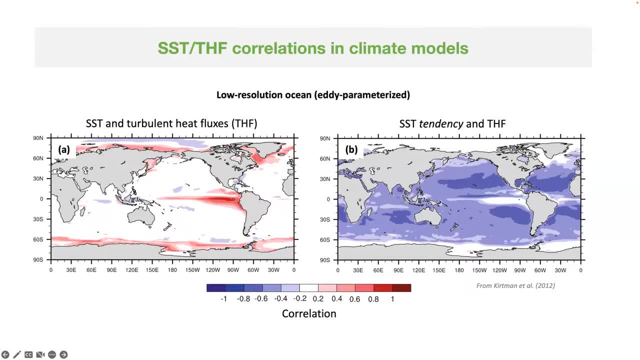 But anyway, in the case of these model, uh the negative system that's consistent must be Never Sorry, Uh, sorry, But anyway, in the case of these model, uh the negative, Um, sorry about this, I think it's gonna slip back and forth. 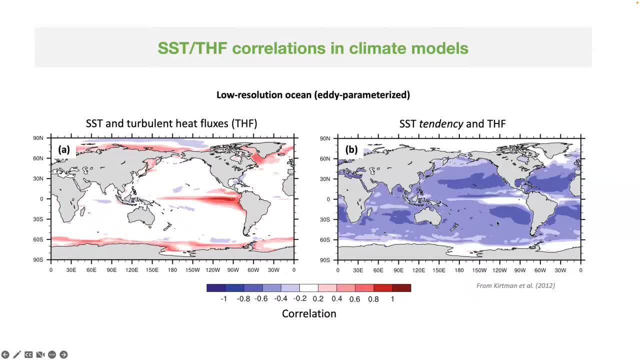 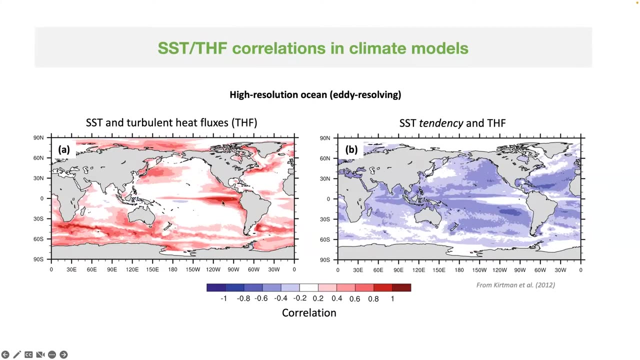 Uh, I apologize in advance. Oh, should have fed the control zero. No, I apologize. correlations indicate that the atmosphere dominates the variability in the exotropics almost everywhere. But this picture changed. It is a simulation configured with a high resolution at a resolving ocean. 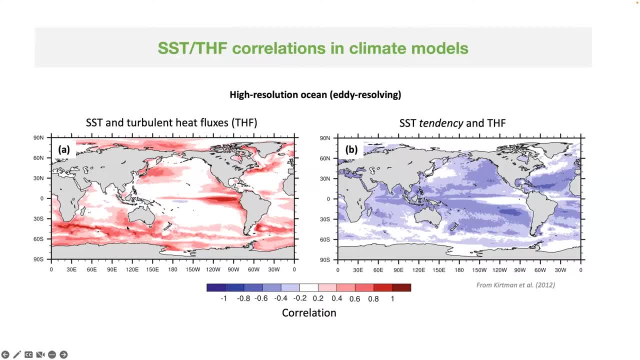 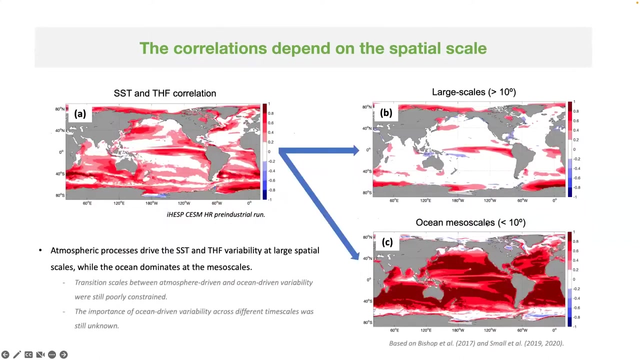 Now, panel A shows strong positive values at regions with strong genicular systems, while B shows very weak or near zero values in the same regions, And this suggests that strong current systems, ocean dynamics dominate variability, although the atmosphere in this case is still dominant at the interior of the ocean basins. 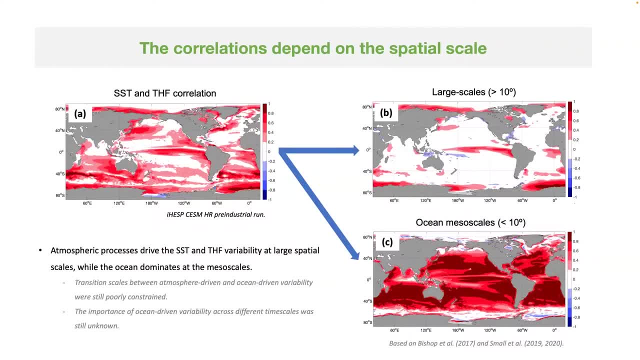 Recent studies also demonstrated that these relationships also depend on the spatial scale that you're looking at, And in this slide I tried to demonstrate this dependence Using a high-res CSM data: data from a high-res CSM simulation filtered in space. 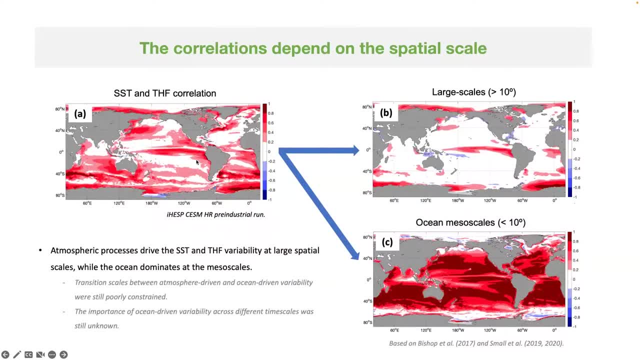 So panel A shows the point correlations between SST and THF, while in panel B I removed variability with scales larger than 10 degrees, And when you filter the data you can see that the correlations dropped to almost zero in both locations And we end up with a map that's very similar to that that is produced by a low-res simulation. 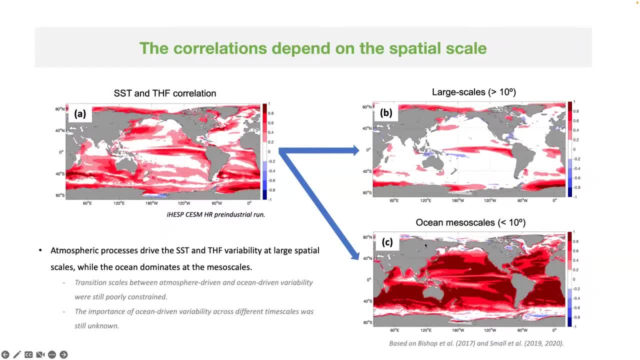 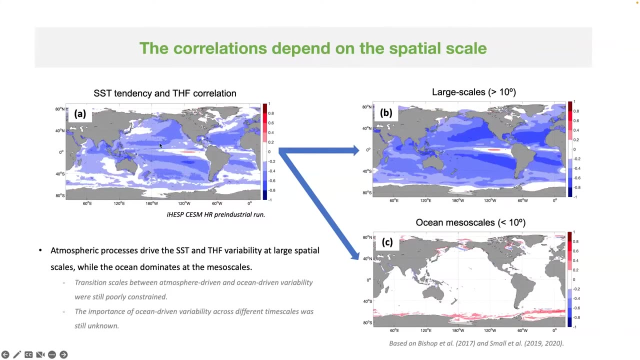 In contrast, if we do the opposite, if we remove variability at large scales and retain only the ocean level scales, we now obtain positive correlations almost everywhere in the ocean. These are in this slide now. These are similar results, but correlations between the SST dependence and the tabulated 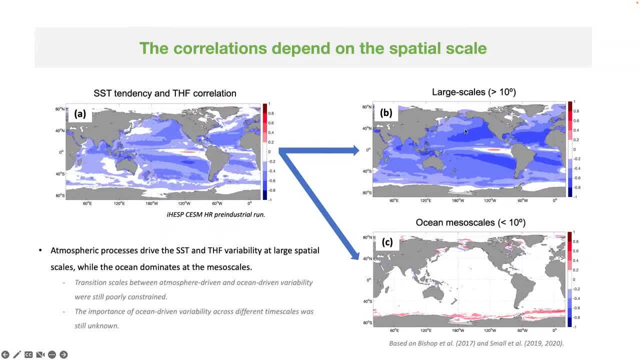 fluxes. And note that when we do so, when we filter to retain only the large scales, the correlations in the core become more negative almost everywhere, while if you do the opposite and retain just the mesoscales, we end up with near-zero correlations almost everywhere. 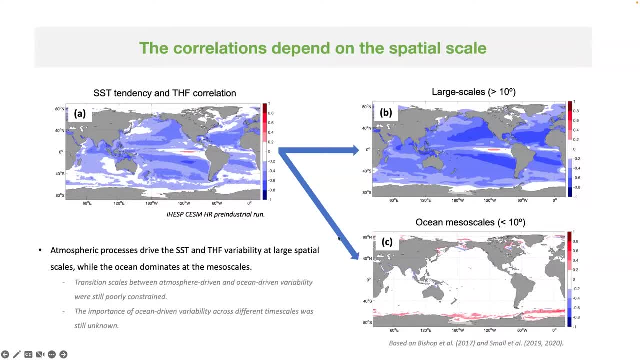 Anyway, These results indicate that the atmosphere controls the SST and reflex variability at large scales, while the ocean processes dominate at smaller scales. However, before this study, those previous results did not constrain well the scales where the atmosphere-driven variability gives way transitions to ocean-driven, nor what 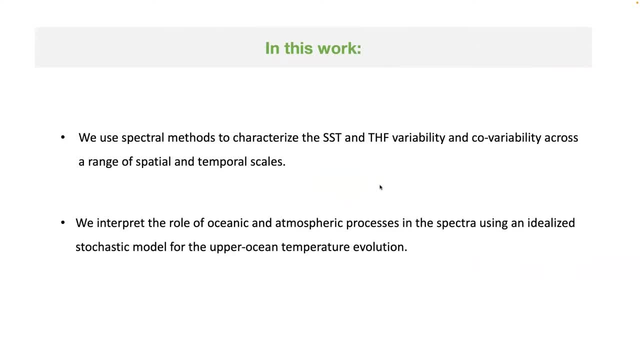 are the time scales where each regime operates. So the main objectives of this study are to determine the influence of ocean in the atmosphere in driving the variability, and to investigate, gain some insight on the physical mechanisms that give rise to this skill dependency, And for that we use spectral methods to characterize the SST and reflex variability and also their 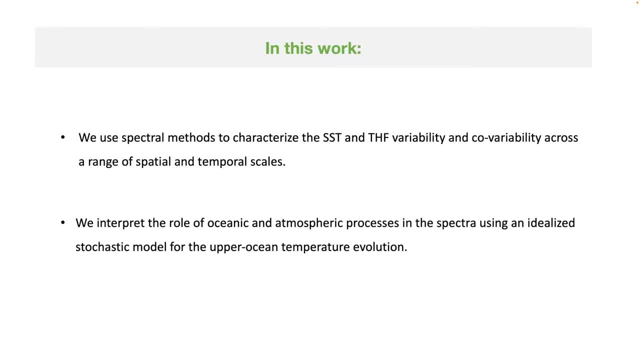 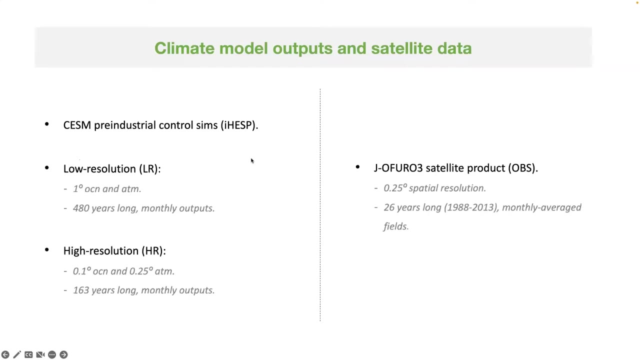 core variability across a wide range of spatial and temporal scales. And we also use a, An idealized stochastic model, to interpret the contribution of the ocean, oceanic and atmospheric processes to the observed spectrum. So I essentially use two CSM simulations. One simulation is low-res, with a one-degree resolution in the ocean and the atmosphere. 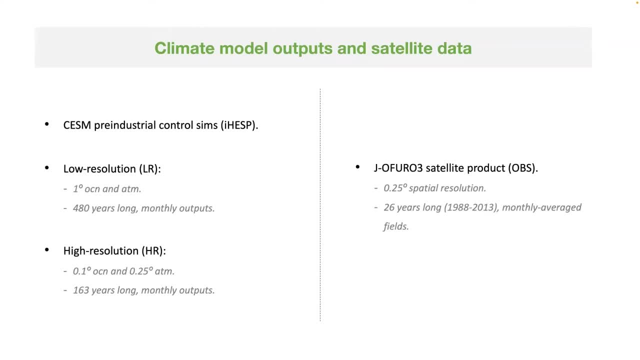 The other one is high-res, with one-tenth of a degree in the ocean and a quarter degree in the atmosphere. Both these simulations, they are pretty long. LR has 480 years of monthly outputs, while LHR has 163 years, And I also contrast those results with those computed using a satellite product, the J-OFOTO3,. 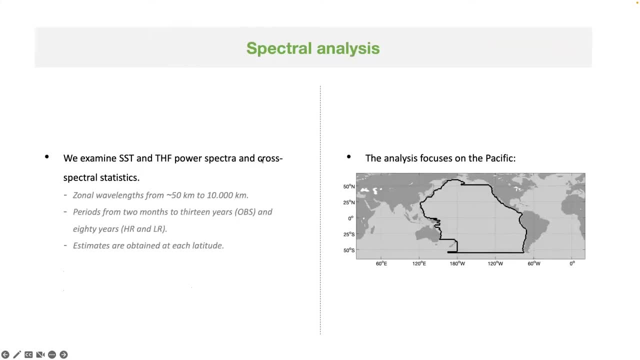 which is 26 years long. This study, I computed the power spectrum of SST heat flux and their cross-section, And I also contrasted those results with those computed using a satellite product, the J-OFOTO3, which is 26 years long. 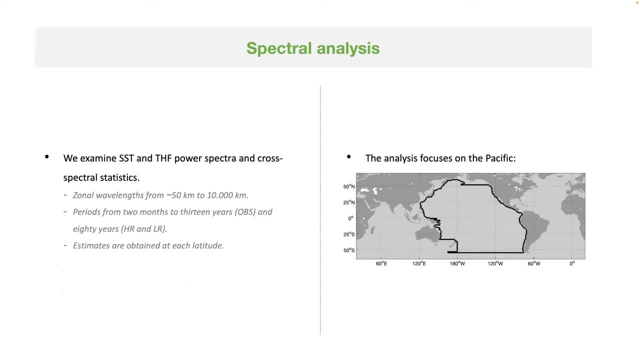 This study, I computed the power spectrum of SST heat flux and their cross-section And I also contrasted those results with those computed using a satellite product. hardware deaths, And I also contrasted those results with those computed using a satellite product. 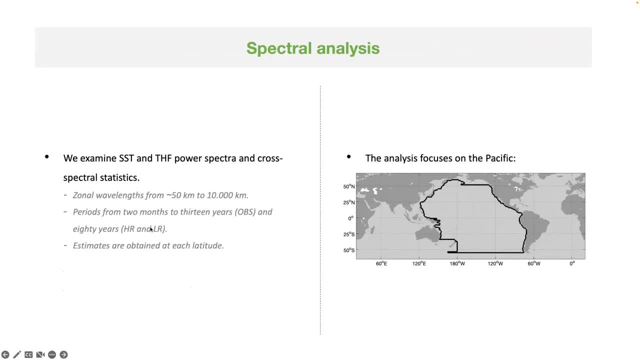 heat flux and their cross-section And I also contrasted those results with those computed using a satellite product heat flux and their cross-section, And there was an idea that we could make tens of millions of doseробux spectra as a Median. 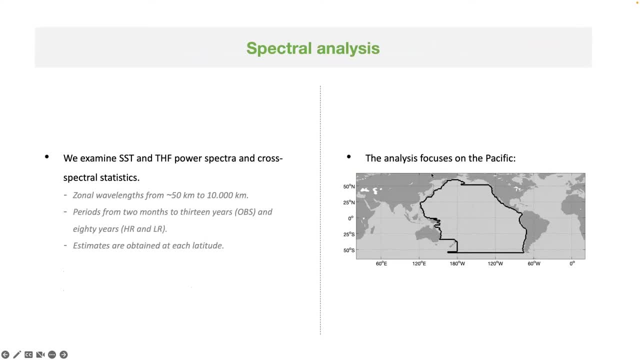 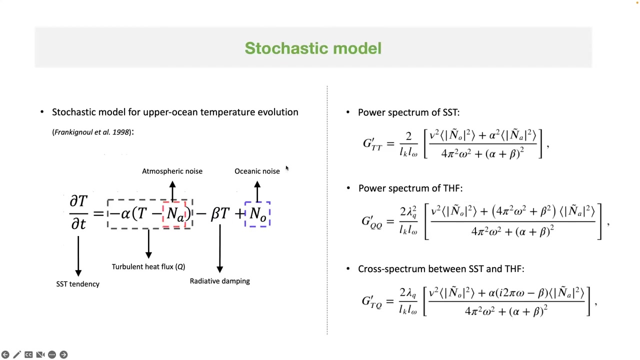 group as a function of zone of wave number frequency. I calculate these spectra at each latitude of a base for the Pacific Ocean that I'm showing here. So I compute the results at each latitude inside this region that's bounded here And to help her interpret the 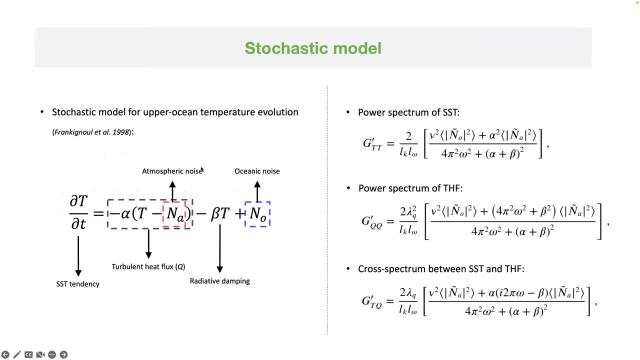 I use a stochastic model, Okay, describing the SST evolution. This model is forced by the noise terms MA and NO, which represent the action on internal dynamics in the atmosphere of the ocean, And it is composed of a turbulent heat flux term that encloses the stochastic atmospheric noise. 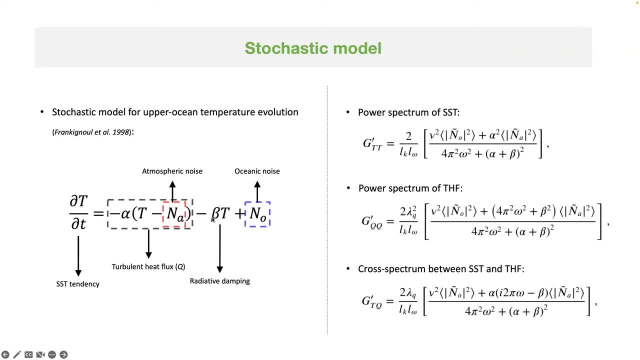 and a radiative damping term that attenuates the SST anomalies over time. Essentially, I solve this model for the Fourier transforms of SST and heat flux and I obtain analytical solutions for the power spectrum and cross-spectrum, which are shown here. I'm showing these equations just to show that all solutions 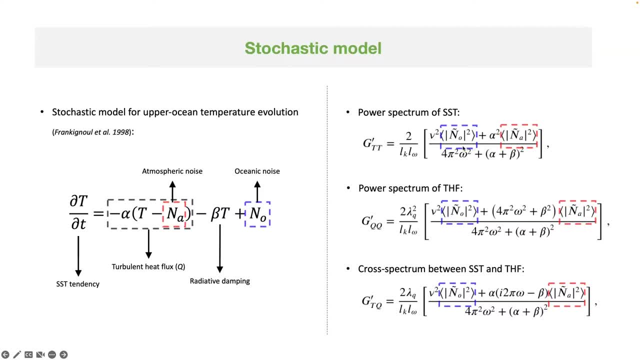 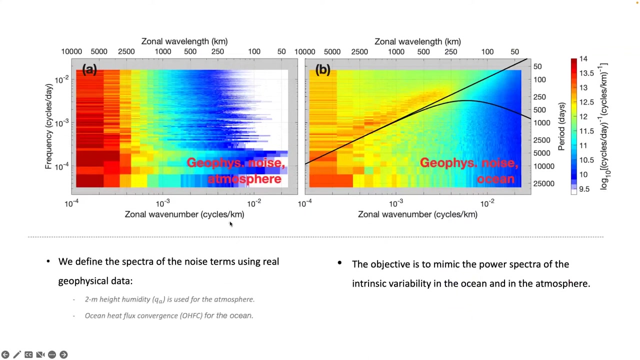 they depend on the noise terms MA and NO And previous studies based on stochastic climate models. they assume they force the solutions using white noise. But in this case I wanted to use noise with a realistic variance distribution, spectral space, And the reason for that is that I wanted to check 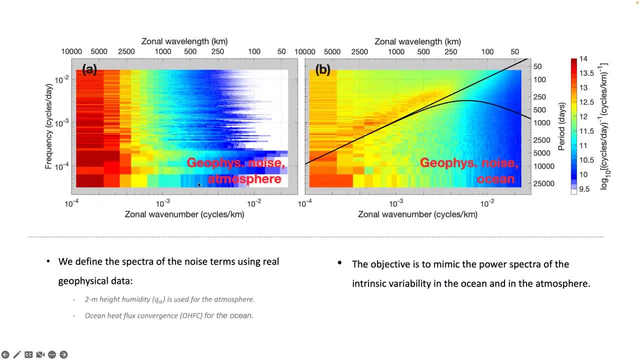 if the presence of structure in the noise could explain the scale dependency of worst interactions that I showed before. And to do that, to generate noise with structure- I decided to define the noise using data from the CSM simulations themselves. So I used two meter height. humidity for NA. 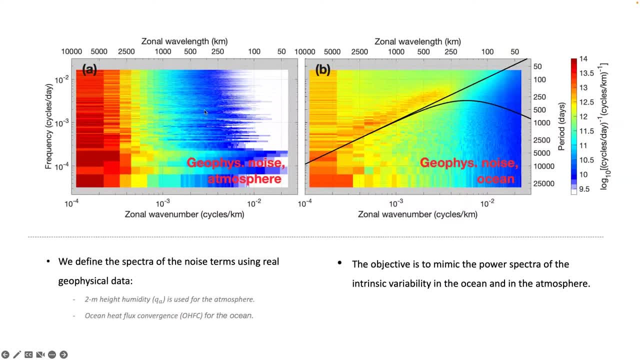 because we found that that was not strongly correlated with mesoscale SST anomalies And we used ocean heat flux conversions for NO, because we know that it is the primary driver of mesoscale SST variability. Essentially, I completed four heat transforms of the signals and plugged them into the stochastic models. 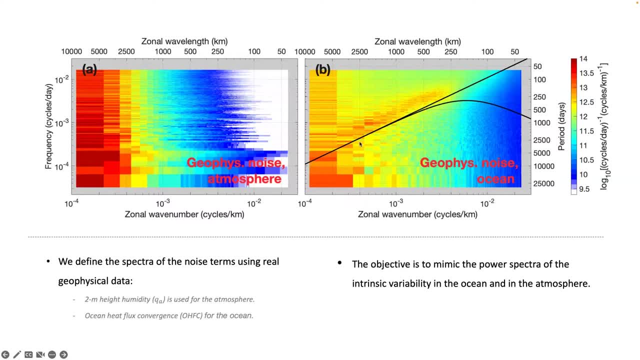 on the solution And I then adjust the noise variance to the correct magnitude by fitting the solutions to the SST he flux spectra from the CSM Pyramids. Anyway, the figure on the slide shows the power spectra of NA and NO as a function of zonal mass numbers. 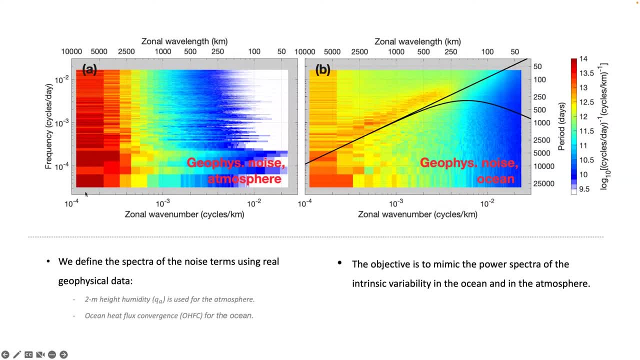 spatial scale and in first person Mkommen. Uh, note that they show structure. They're not purely right. Uh, that was certain wise. Uh. it is approximately white in frequency space, But it is strongly red in sort of with number with much more power over large wavelengths. 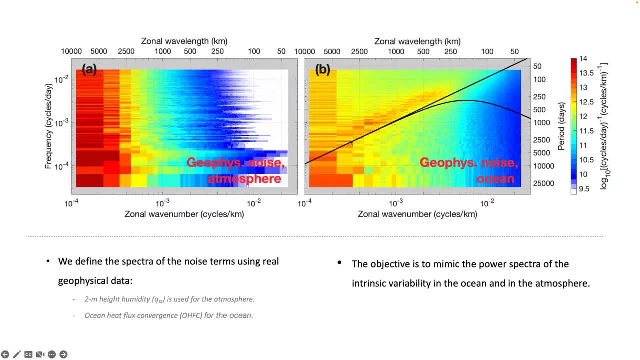 And you can see that the ocean noise. it is a bit different, Uh. it is also reading wave number space with more, more variants of large skills, Uh, but it shows more variability, Uh, close to these lines here, which are the special relations of uh. 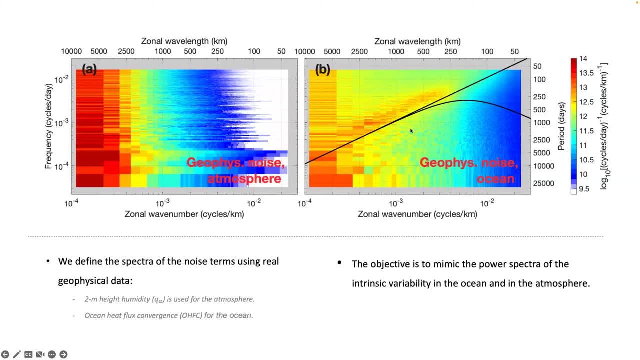 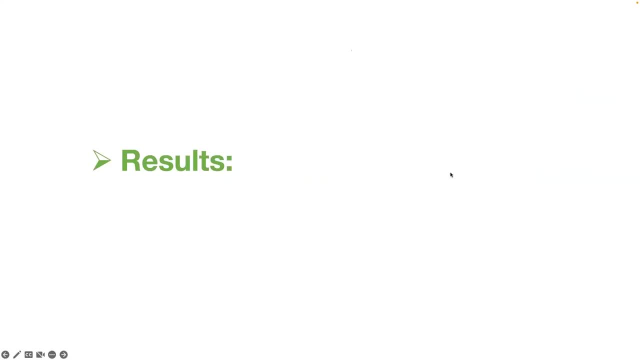 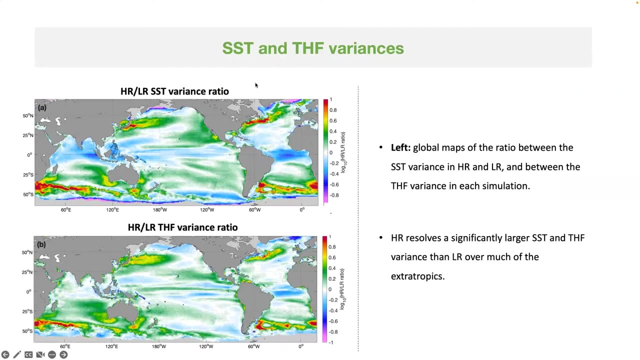 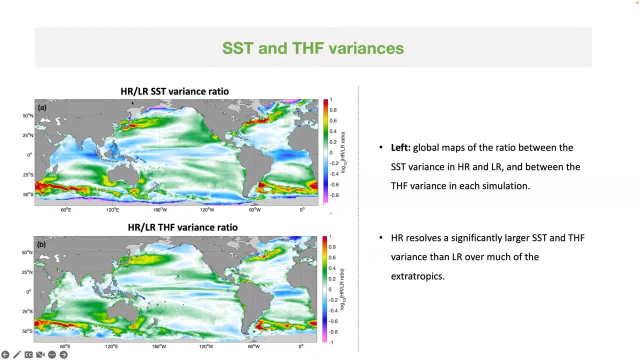 Uh, then a ways for Penalties for the chef. uh completed the variance without uh, without the system cycle. So there are anomalies about the, about the mean and the seasonal fluctuations, And what it shows here is that HR results much larger variances than a line. that's a topic for both uh. 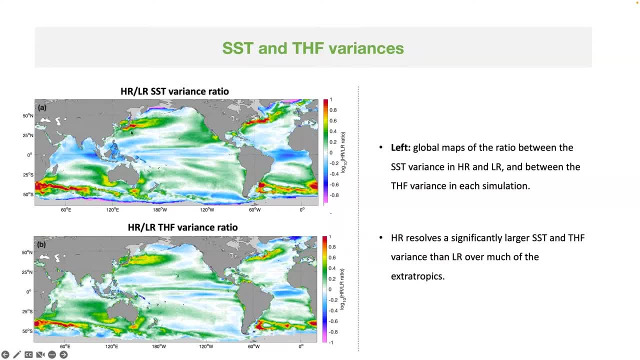 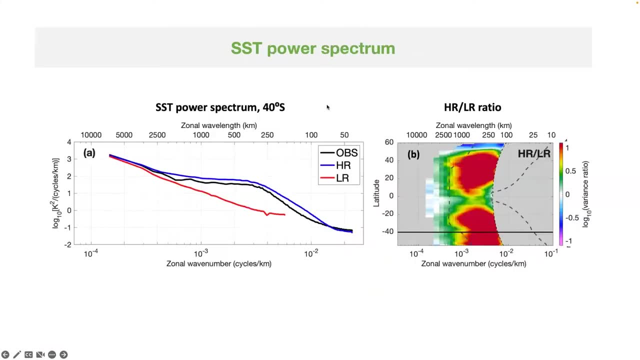 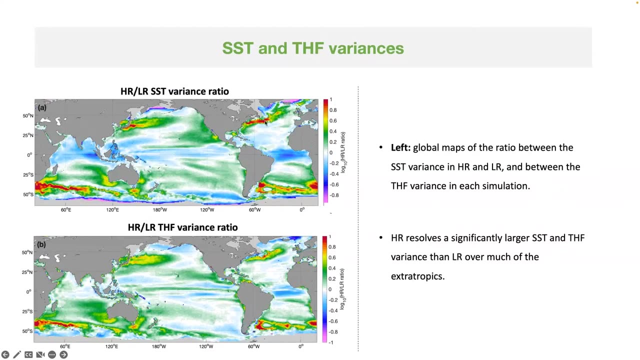 For both quantities notably coincide with uh, Uh, current, uh, current systems- And note that the color skill he is logarithmic, Sorry, Uh. meaning that a value of 1 means that HR has 10 times more variance than uh. a lot. 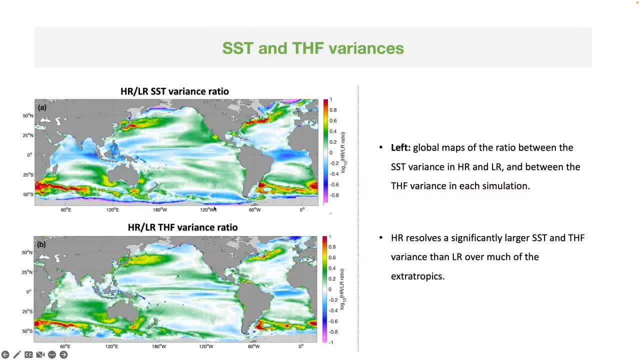 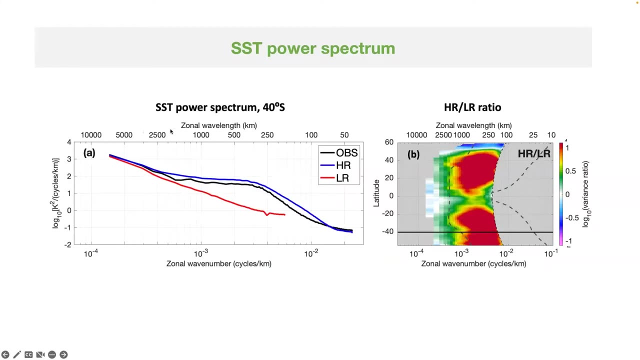 And the maps are also very similar with each other. uh, which is consistent from the interpretation that they try. accessibility ability driven by ocean processes is driving response. Now, uh, here I'm showing the spectrum as a function of uh. I was only with number uh, just for us to see the results for the blend, which is very similar to these. 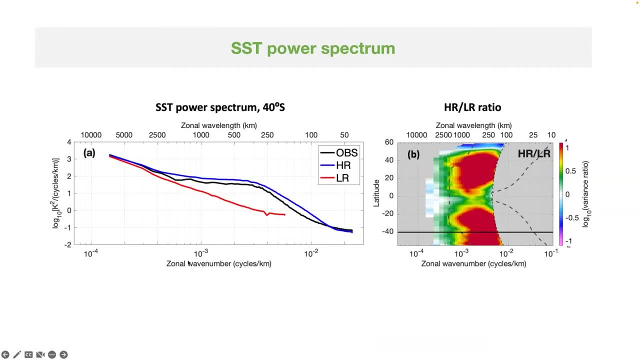 And then we show estimates for for itself in the Pacific. Where are the black lines for from the satellite observations? Uh, blue is for HR and red is the Oh wow. Okay, That's cool. Here goes from about 75,000 kilometers to 40 kilometers. 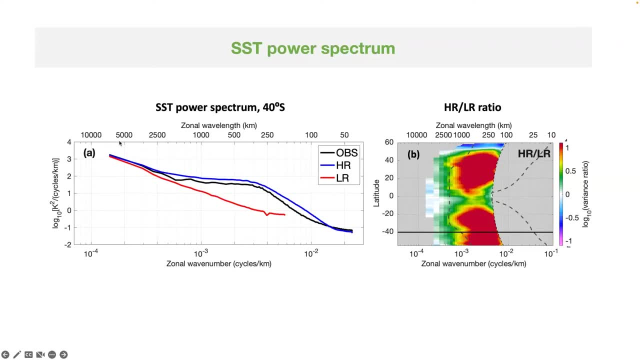 Uh, note that All they the set, they resolve similar uh variability, Especial skills larger than 2500oki longers. But as you go towards model skills, notes that the verse remains high in observations in HR. Well, it just keeps the gele twists. 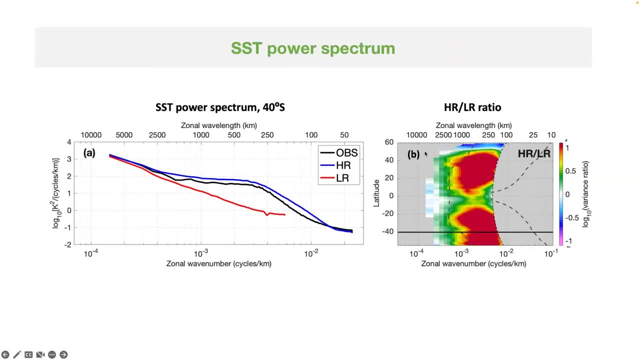 So Tenno A is just for 40 South. Tenno B shows the ratio between the variances in HR and LR, but as a function of latitude. This black line here marks where I got these results from. Note that this difference in variance between HR and LR is of course not just at 40 South but at most latitudes in the exotropics. 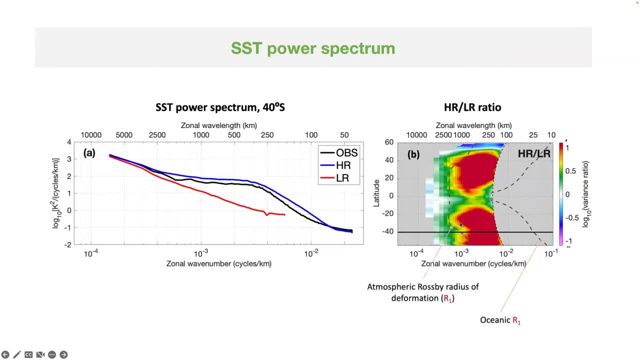 And for reference these dashed lines here, they represent the Rosby radius of deformation in the atmosphere and in the ocean And it shows that the most significant difference between HR and LR- it of course has scales smaller than the atmospheric Rosby radius. 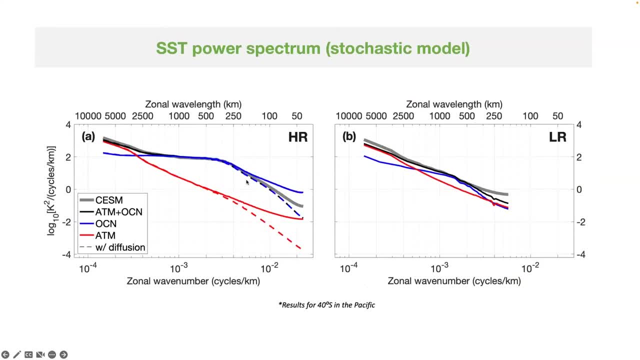 So this slide shows the corresponding estimates obtained using the stochastic analysis. This is the stochastic model representing estimates for HR and LR. Here the gray lines, they are the power spectral computing using CSM data, While the blue lines are stochastic model estimates computed using geosolution noise. 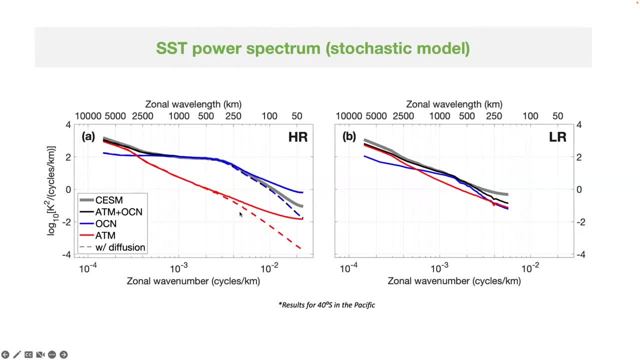 and the red lines are estimates obtained using atmospheric noise. The black lines that you can barely see here are the sum between the blue and the black lines. In Tenno A we can see that the atmosphere-driven component significant at large scales, The curvature is. that allows the ocean-driven. but sorry about that. 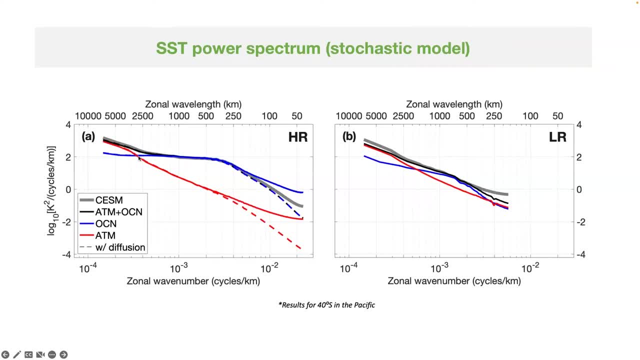 The atmosphere-driven noise is very strong at large scales, but it just diminishes steeply as you go towards smaller scales, and this steep decrease is what allows the ocean- driven temperature modulation to prevail, And And this happens at fairly low wavelengths, close to 2,500 kilometers in this case. 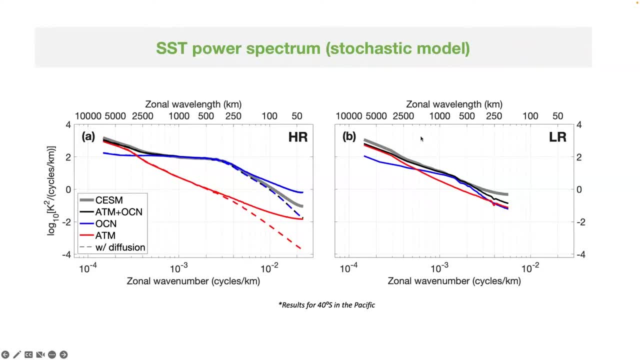 TenoB is for the low rest. We see that something similar happens, but the ocean-driven component, the blue line, is much weaker than the HRI, While the atmosphere-driven component- actually it's pretty similar in magnitude to that- resolved. 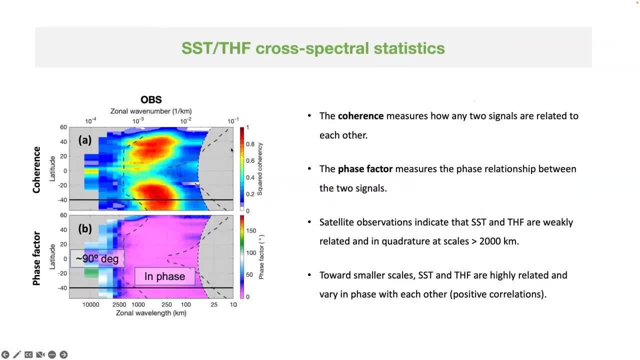 by HRI. So now in this slide I'm showing the cross-spectrum statistics between the SST and heat fluxes as a function of latitude, and first showing estimates from satellite observations. TenoA shows the coherence, which is a quantity that estimates how SST and the heat fluxes 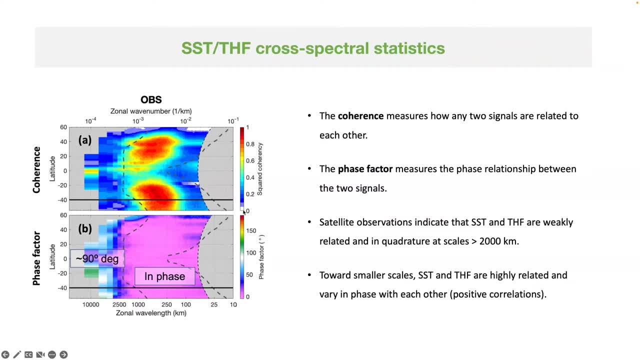 are related with each other. It varies from zero to one. If it is zero, it means that they are completely unrelated. If it is zero, it means that they are completely unrelated. If it is equal to one, it means that they are very together. they are highly related. 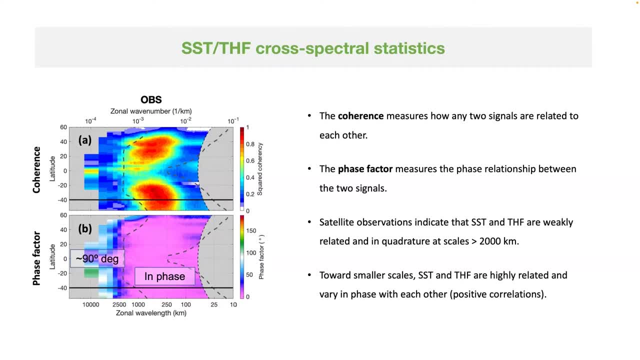 And the bottom panel shows the phase factor, which measures the phase relationships between both signals, And you can see that at large scales we see weak coherences associated with 90-degree phase. However, as you go toward the small scales, the coherence increases and you have a band. 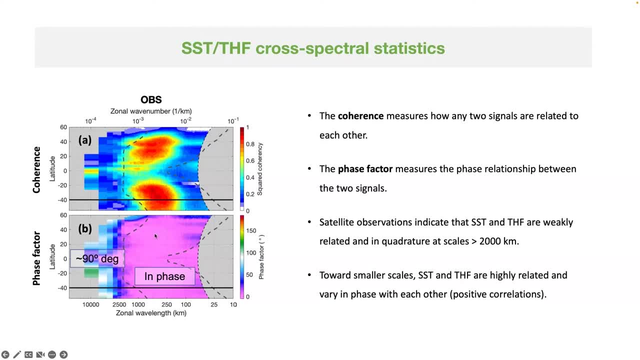 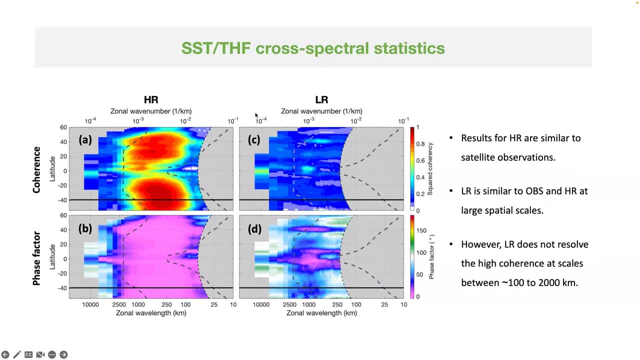 of high coherences here, while the phase goes near zero, And these are corresponding estimates for the high-res and low-res simulations. HR is very similar to OPS. ELLAR does show similar characteristics with ELLAR spatial skills, but it notably misses that band of hyper-res that's present in the other datasets. 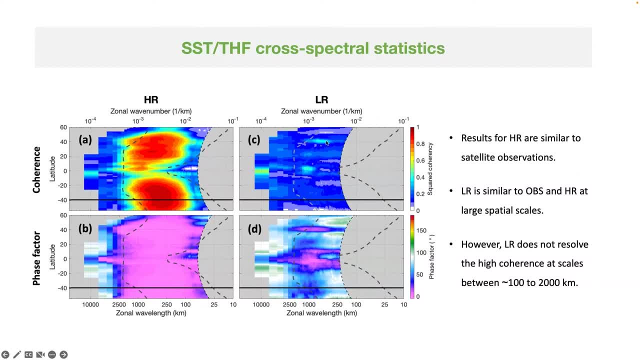 Note that ELLAR shows slightly larger coherences near 40 North and in the tropics coincide with small phase angles. So to me it says that ELLAR even tries to do something similar to HR and OPS, but the signal is much weaker. 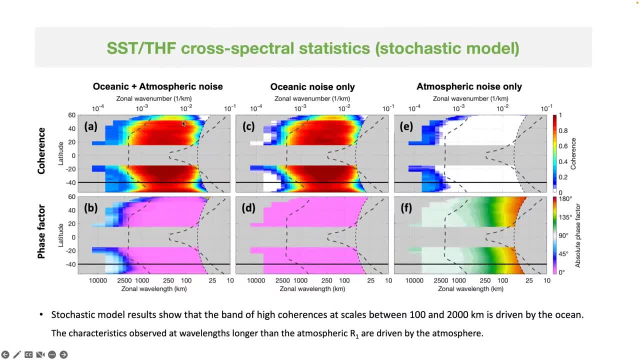 And here in this slide I'm showing stochastic model estimates including the combined effects of both ocean and atmosphere noise. I'm asking latitudes close to the equator because the stochastic model is not there, But we can see that It resolves similar characteristics than the satellites and high-res results. 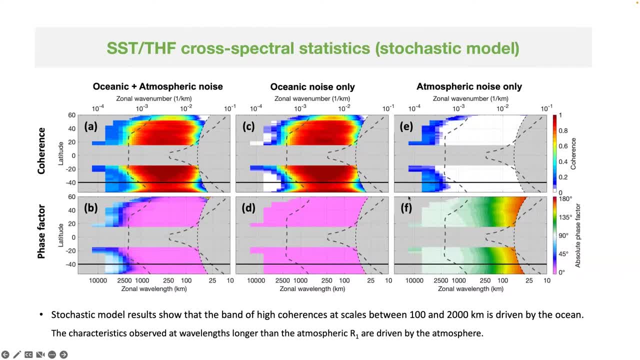 If you go to the other columns, I separate the influence of ocean noise and atmosphere noise And we confirm that this band of high coherences reflects the action of ocean processes, while the characteristics of large scales it arise from the action of the atmosphere. 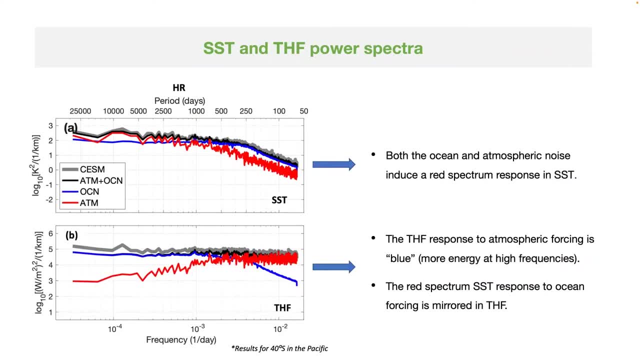 And we can see that the stochastic model estimates obtain as a function of frequency. also just for 40 South in the Pacific and in this case just for the HR run. PNOA is for SST, PNOB is for turbulent refluxes. 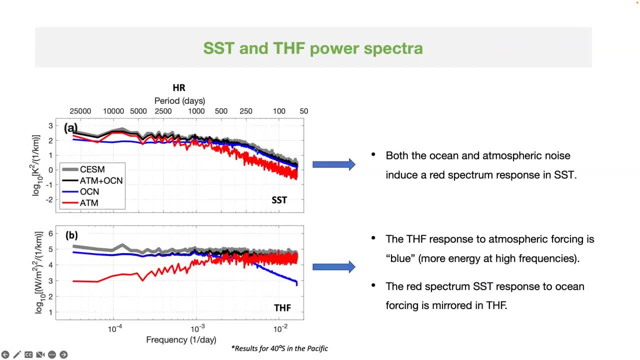 The gray lines are obtained with CSM data, while the blue and red lines are stochastic models made for the ocean and the atmosphere noise. Starting with SST, PNOA, We see that ocean noise produces more substantial variability at periods shorter than about 500 days. 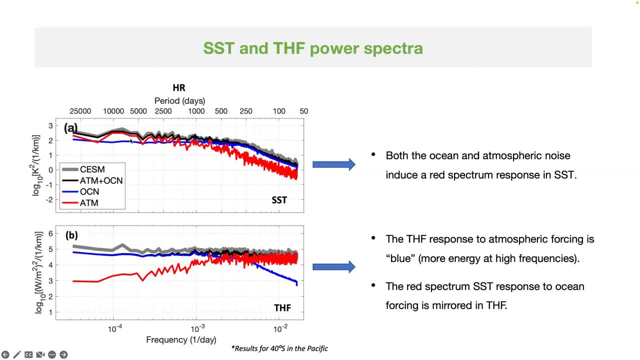 But as you go towards longer periods, the variability induced by the ocean in the atmosphere. they become more or less comparable, although the atmosphere-driven component is stronger here. In any case, you can see that both the ocean and the atmosphere produce more, larger SST. 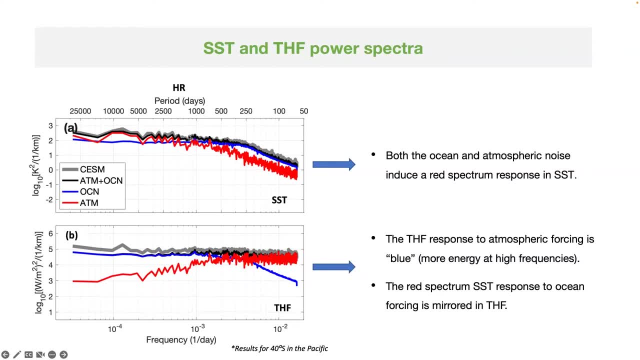 variability at low frequencies And in the red spectrum. it is well-known that the atmosphere drives this kind of response to stochastic forcing, but here we find evidence that the ocean noise can do something similar, And looking at the heat fluxes, we find that the atmosphere controls most of the variability. 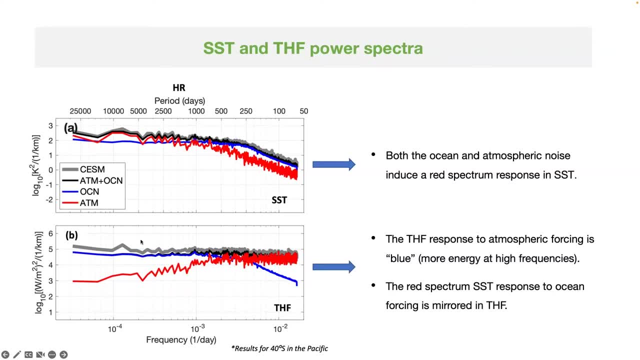 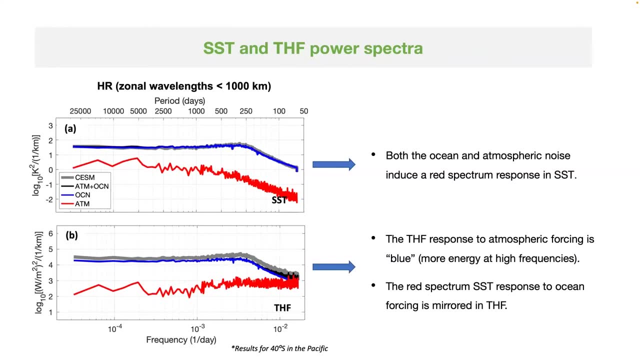 at higher frequencies, while the ocean controls variability at low frequencies. And to double-check our conclusions of the influence, Let's see The influence of ocean processes. we can filter out large scales and then we compute the frequency spectra And when we do so, note that we obtain spectra both for SST and turbulent heat fluxes, with. 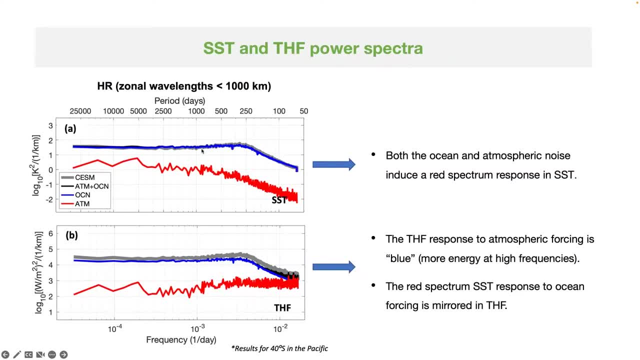 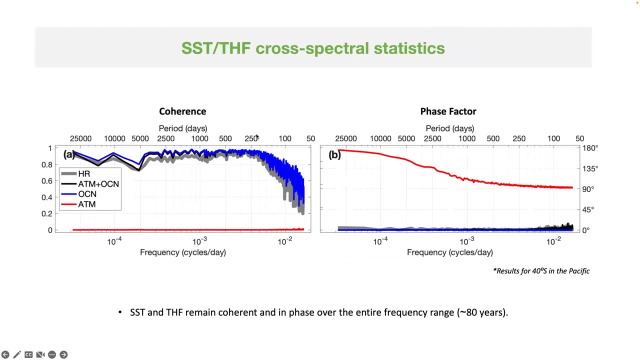 very similar shapes, And the blue lines here indicate that most of the variability at these scales are driven by the atmosphere, And we can see that the atmosphere is quite close to the ocean noise. Now, this is the coherence between SST and THF that is predicted by stochastic model. 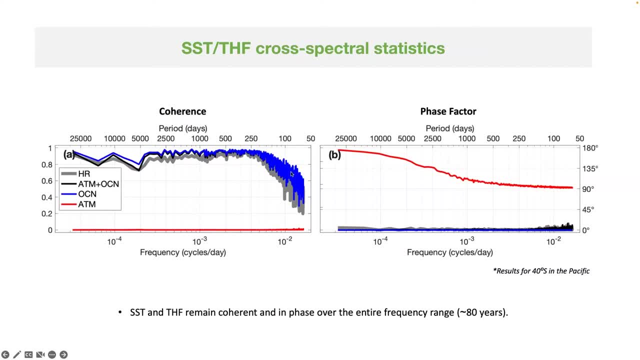 This is also for spatial scale smaller than a thousand kilometers, And these results indicate that SST and THF. they remain coherent and in phase over the entire frequency range that we are analyzing, which goes to about 80 years, And this model confirms that the highly coherent signal arises from the action of motion processes. 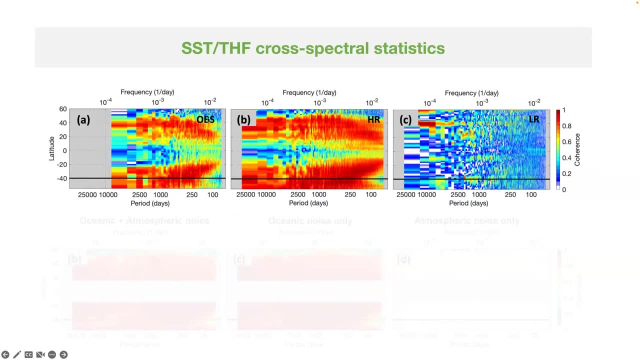 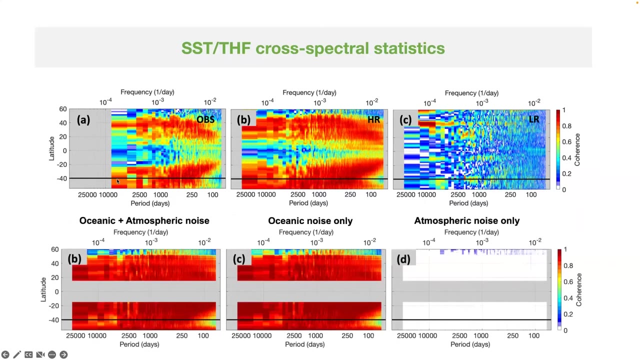 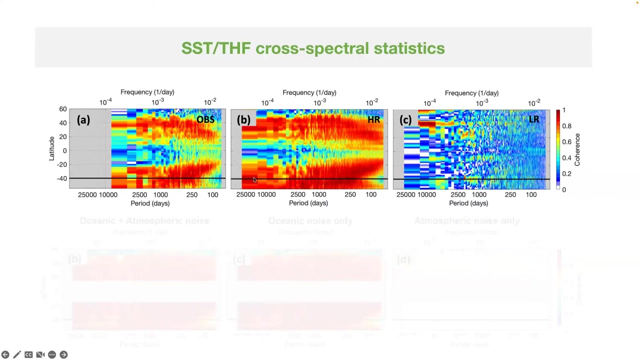 Now this is our estimates, not from SOC-SK model, but for observations HR and LR. This is just the coherence, And again we see that this highly coherent signal, they, they are present in observations HR results. a very similar feature, although it seems a bit stronger than the Schomburg observations. 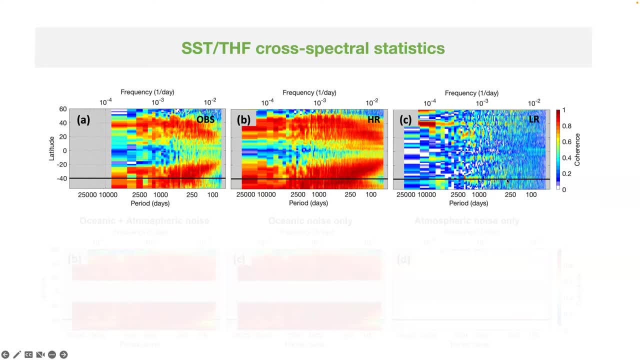 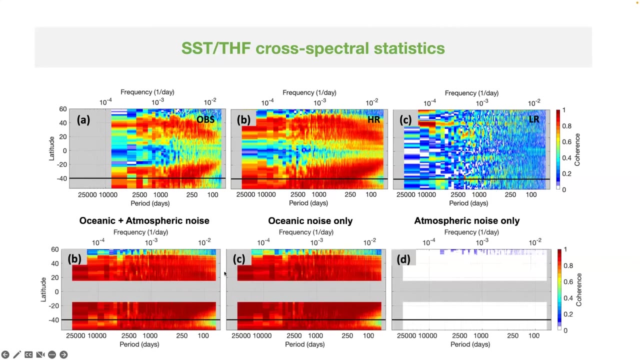 While LR just showed this very noisy signal which indicates this is dominated by noise essentially. And the bottom is just the corresponding estimates obtained using the stochastic model, which also shows that these high coherences are coming from the influence of motion processes. 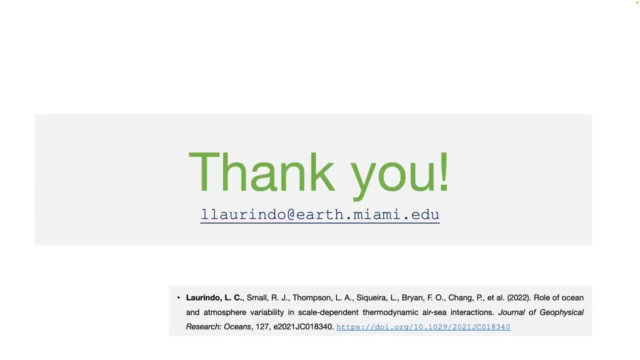 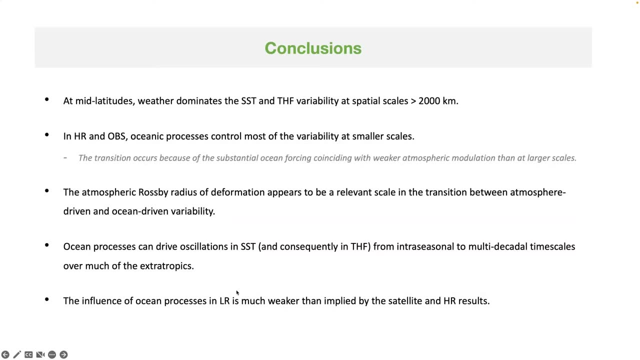 So the conclusions We found in this study that the atmosphere dominates the SST and THF variability at spatial scales smaller than or about 2,000 kilometers, That in HR and observations ocean processes control most of the variability towards small scales. The ocean can prevail at these scales because ocean forcing is strong, while the atmosphere forcing is much weaker than what we observe at large scales. 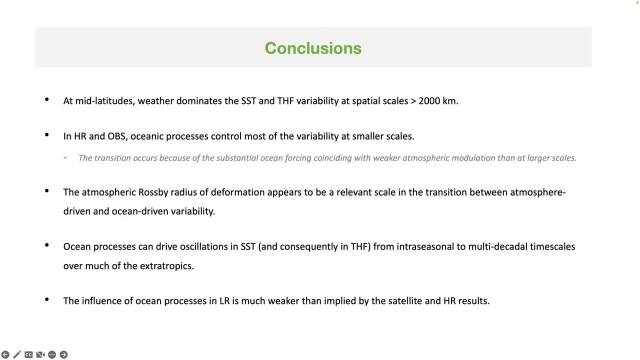 We found that the atmospheric cross grades of the formation seems to be a relevant scale controlling the transition between atmosphere driven and ocean driven. So we found that the atmospheric cross grades of the formation seems to be a relevant scale controlling the transition between atmosphere driven and ocean driven. 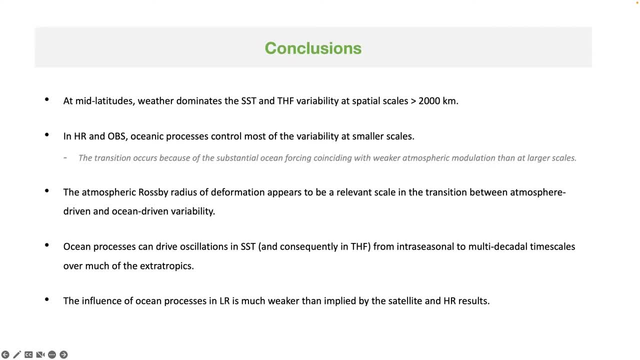 So we found that the atmospheric cross grades of the formation seems to be a relevant scale controlling the transition between atmosphere driven and ocean driven, Although we still don't have a good explanation of why that is the case. We found that ocean processes can drive us oscillations in SST and on therift fluxes, with time scales ranging from intercélusons to moments decadal over. of these syst textbookics: 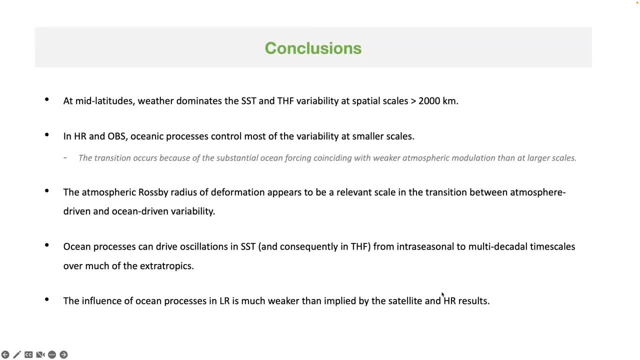 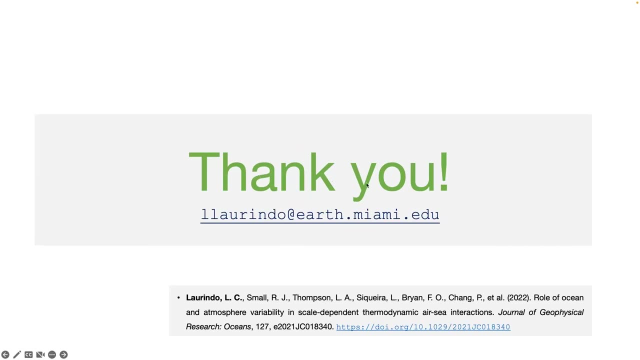 And finally, we find that the influence of motion processes in the LRinned simulations is much weaker than that implied by satellite and high-resolution. Thank you for going over these results. Thank you for going over- sorry for going over time and thank you very much. 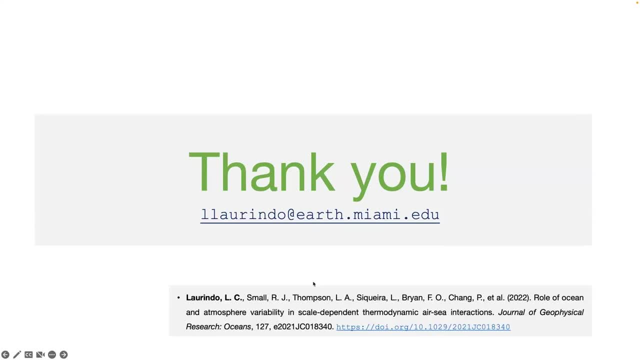 Showing here the- my email, if you would like to contact me, and also the reference for the study. Thank you very much. Thank you very much. Yeah, yeah, Thanks, Lucas, Hey, Michael, Yeah, so I just wanted to thank Lucas and open the floor for comments, if you can raise. 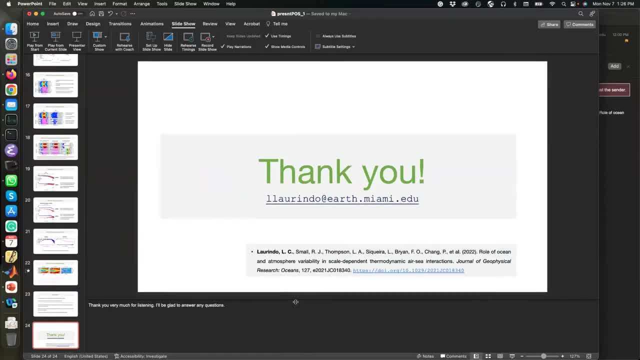 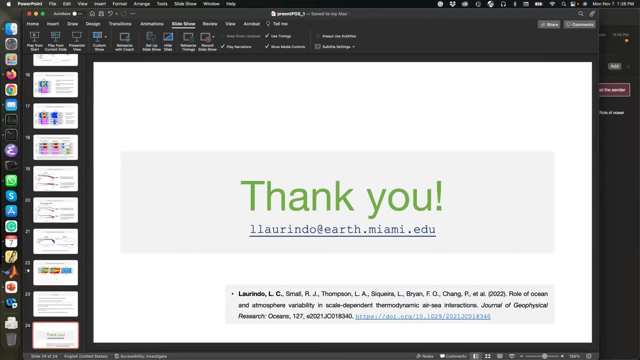 your hand in the chat feature Irana. I'm sorry, Just a silly technical question, because I- since I haven't done that before- When you do your- when you do your correlations, how do you select for- Yeah, For- spatial scales larger versus smaller? 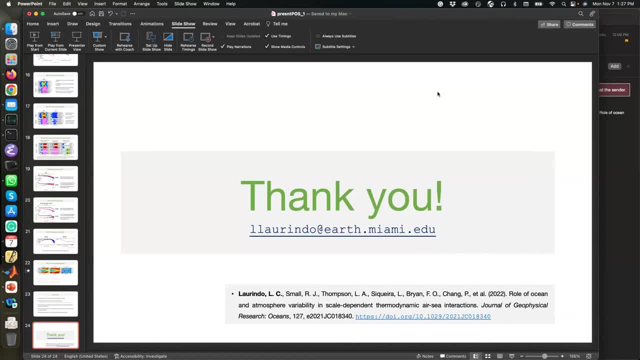 I guess, the same way that you do it for- I mean, I know how to do it for time. How- sorry, it's just silly technical-. Oh no, no, not at all. I use a spatial filter, and the same way that you can filter the signal in space, you can. 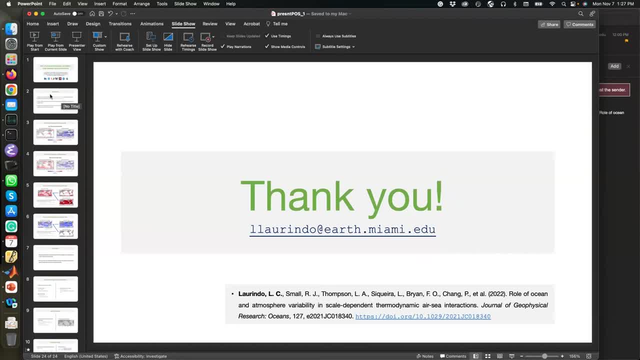 use like a- like a box- moving average filter to just to- a 10-way filter. You can do the same in spatial scale, Spatial fields. So it's as if- it's as if you're averaging over everything smaller than- than you know. 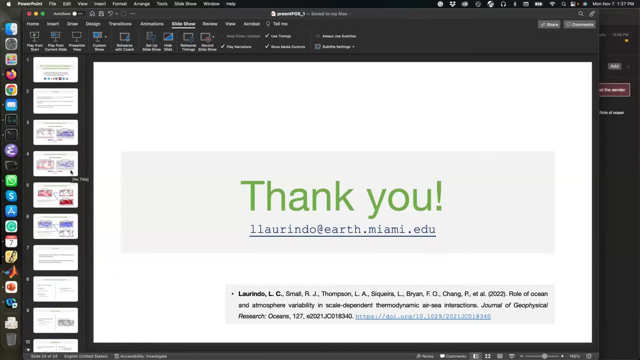 if you have a thousand kilometers by a thousand kilometer, is this like, vaguely speaking, like you're averaging inside this box? Yeah, yeah, We can do this Like this is the easiest way to- to select, Yeah, To select the scales, but when we were developing this research, we found that it's not very. 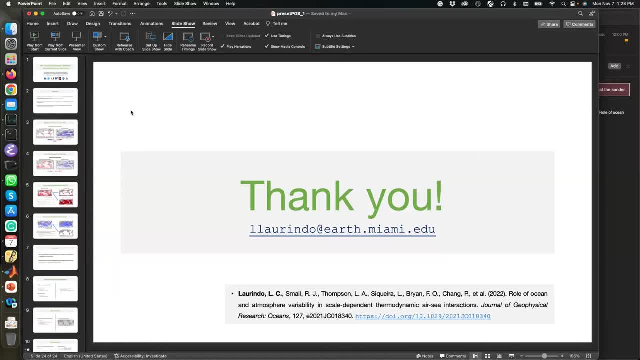 easy to interpret what scales are being filtered, you know. So we- we try to use a better filter, like a Gaussian filter in space, just to- so we can reselect what scales are retaining-. we are retaining Mm-hmm. 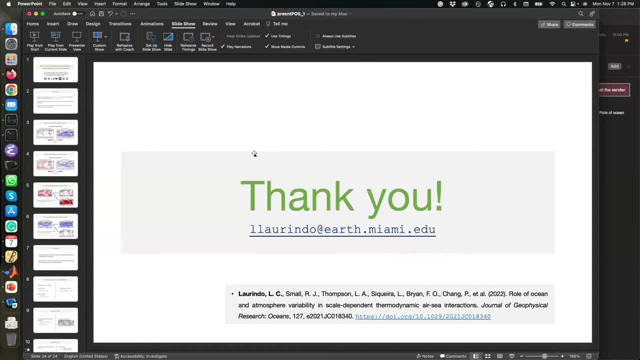 Mm-hmm- Sorry, It's- Mm-hmm, I hope I- No, no, no, no, Yeah, yeah, yeah, It's good, It's good, It's good. And then you can do it selectively. 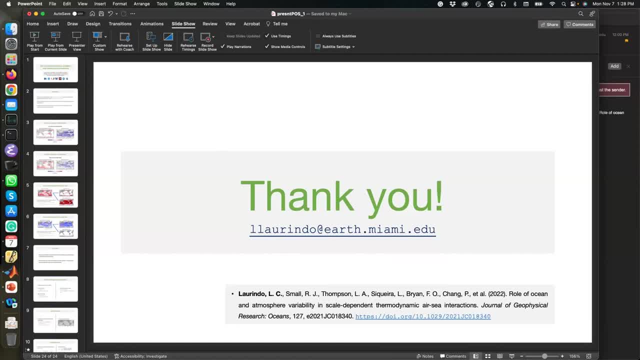 I see, And then your picture was showing, yeah, that the-. can you explain once more? the one where you have both the atmospheric Rossby radius of deformation and the ocean one? Sure, What was the meaning there in the end? Yeah, 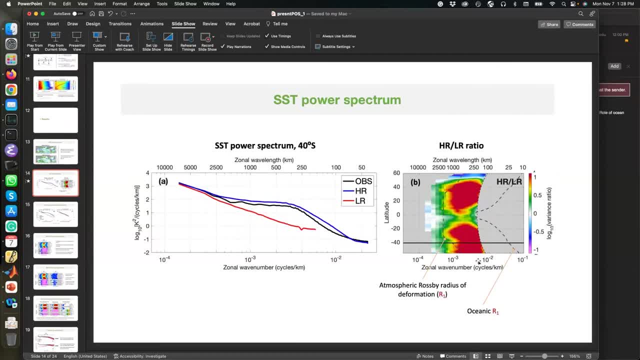 The one on the right. Yeah, This is the power spectrum of SST as a function of zonal wavelength Mm-hmm, And I'm computing that for every latitude within the Pacific. And then I just made a plot like this one: 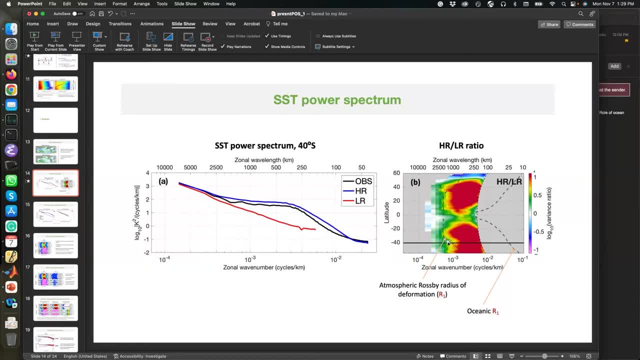 Mm-hmm. I'm showing the ratio And what I'm showing here, the Rossby radius of deformation. So I'm not filtering the data here, I'm just computing the spectrum as a function. Oh, I see, Yeah. 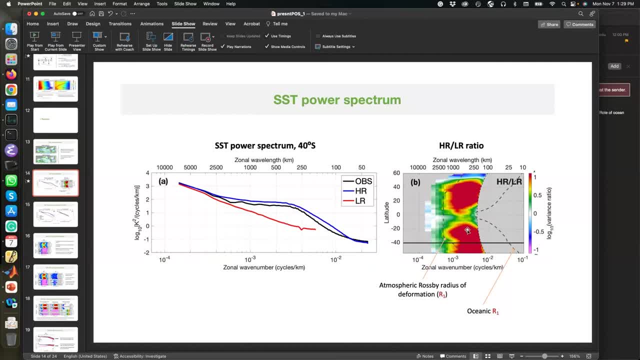 To generate this kind of visualization I don't need to filter, Just compute the spectrum. And yeah, Here it's showing me, like the difference between variances, like the scales where each model of- where the variances are different. Yeah, 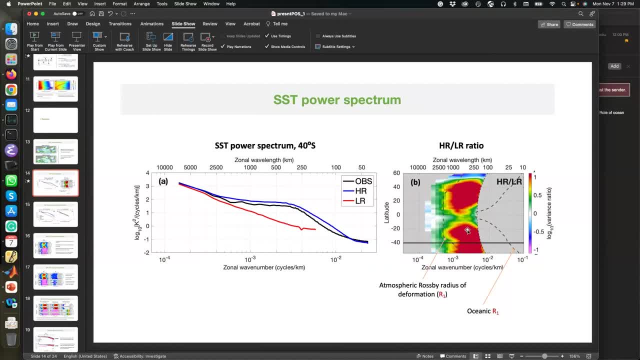 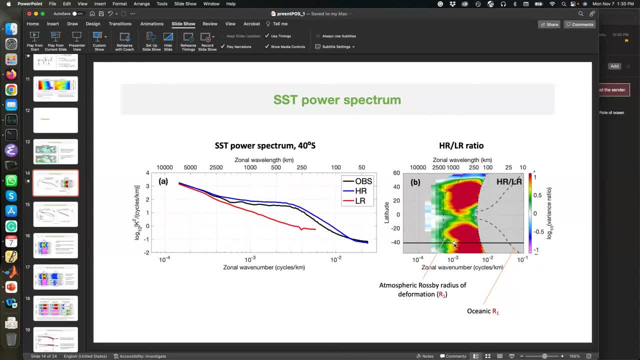 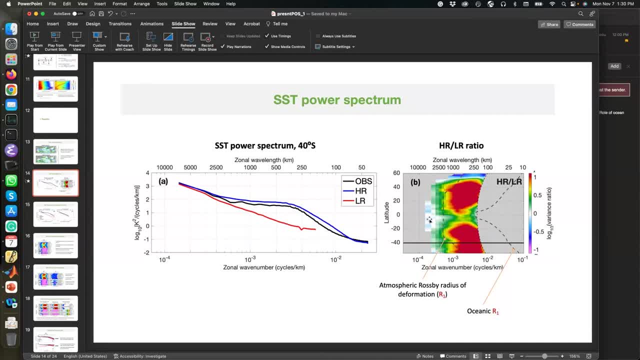 Mm-hmm. OK, this is driven by ocean noise or atmosphere noise, And what we found is that most of the variability at large scales, the SST variance here, is driven by the atmosphere, by atmospheric processes, But as you go towards scales that 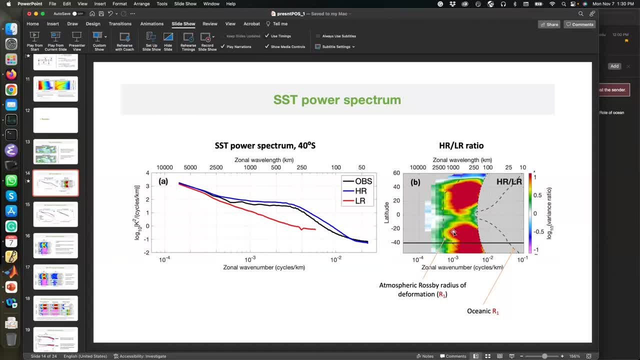 are smaller than the forms of variability, smaller than across radius of deformation in the high-res model and in observations. the variance here is driven by ocean processes And the reason that the low-resolution model does not resolve this like has so little variance over these scales. 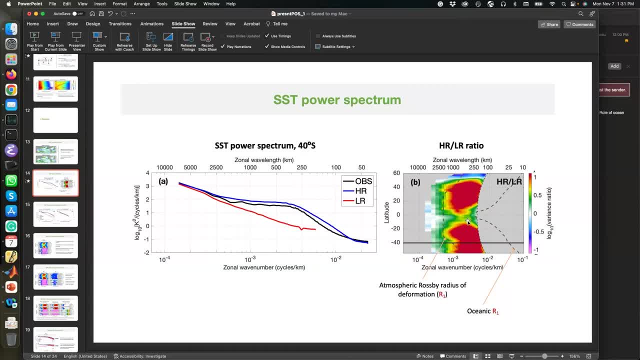 because that's a scale that variability is very weak, So it does not really move heat around as much. Mm-hmm, got it OK. we do have a couple of other questions as well, Jimbo. Oh yeah, just quickly. 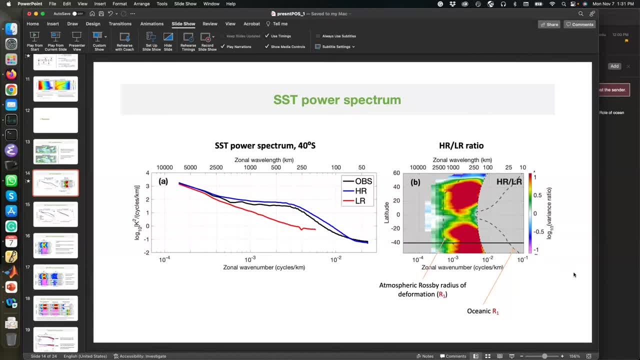 Yeah, thank you very much, Lucas. This is great work. I just have a question. In general, you have shown the influence of the high-resolution simulation both in atmosphere and ocean in the air-sea coupling process, But, as we know, climate model is mostly low-resolution. 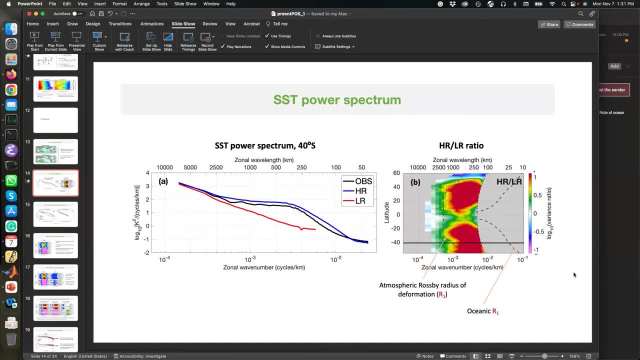 How to really solve this problem, either through polarization or other method. what is your take and what is the community's proposed approach for addressing this question? One solution is just go high-res, you know, just to alleviate these biases. But there are. the community even been talking to colleagues. 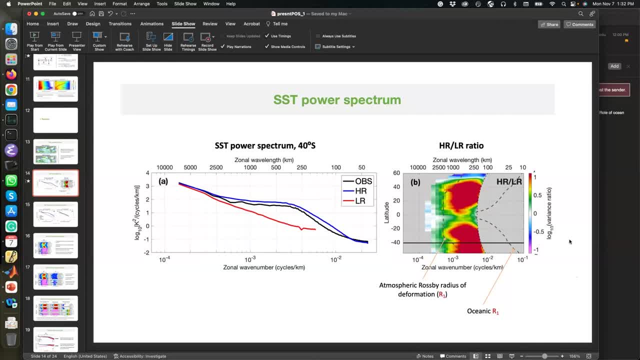 to help, And so you can go high-res to be able to do this. But I think the way we can do it is, you know, we can do it with a little bit of roughness, So we can really do it with a little bit of roughness. 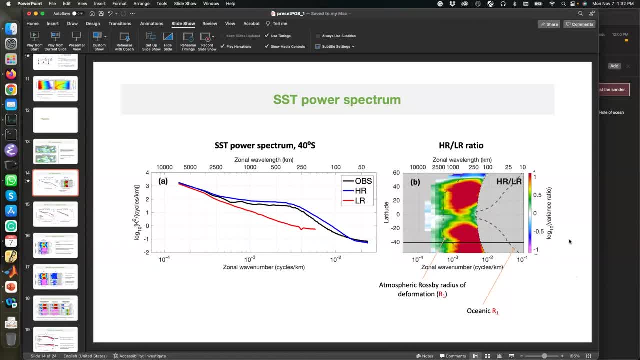 But it's not clear how to do this yet, as far as I know, using parameterizations. But I don't know. I think that's possible, Thanks. Thanks, Mike Sergei. did you want to ask your question or make your comment? 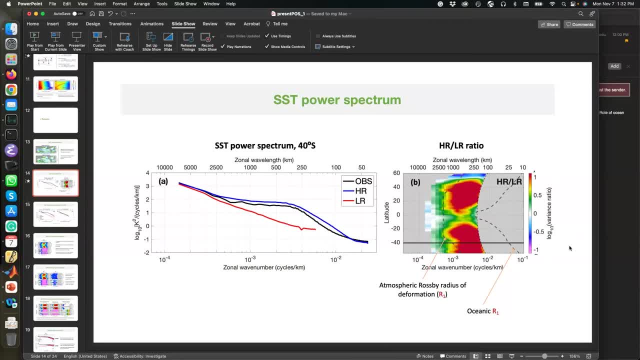 I have a quick question. When you were comparing the HR to water, the HR to low resolution variants, you focused on the places where HR had more variants, but in several cases in the options the opposite was true. Can you comment? why would low resolution run?